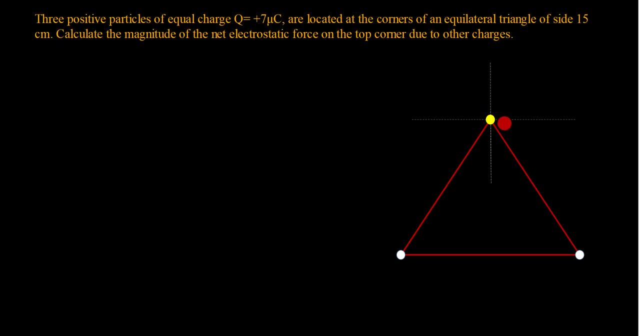 start calculating how much the total electrostatic force generated is Calculated by this charge and this charge on this yellow charge. So first of all I can say: I have here, let's activate the. I have a 15 cm distance here. 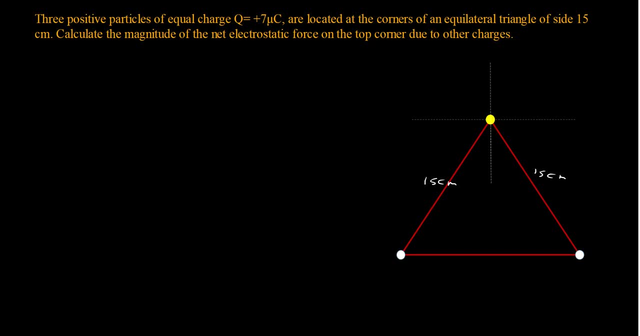 and another 15 cm distance here. I will call this charge here as Q1.. This one will be our Q2, this one here will be our Q3.. Now to start the calculation. we're using Columns Law, which is KQQ over the distance squared. Now to find the force generated on charge. 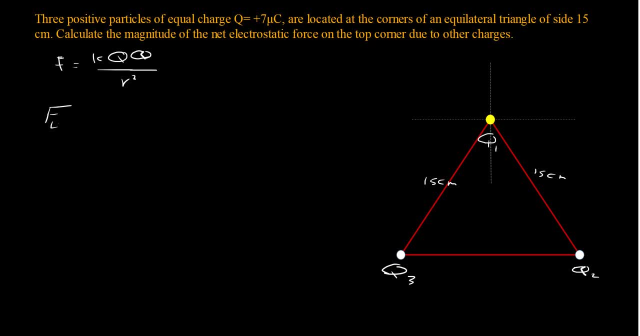 1, because of charge 2,. sorry, let's erase this. Okay, Let's erase this part here. So make it more clear. The force generated on 1, because of 2, is simply say 8.9,, 10 to the power 9, multiplied by 7,, 10 to the power minus 6, and all squared. 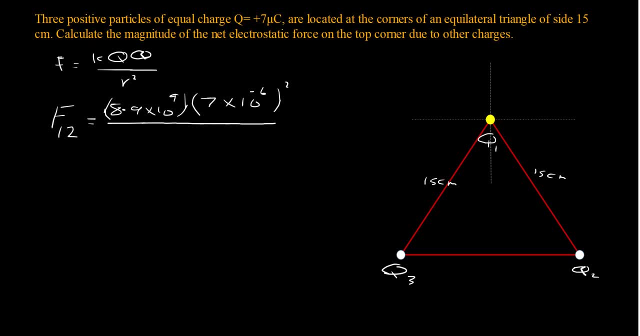 Because all the charges are equal And we divide all this on the distance, which is 15,, 10 to the power minus 2, we have to convert it to meter And it's a square. Doing the math that will give us 19.4 N. okay, Now, before we continue with the calculation, 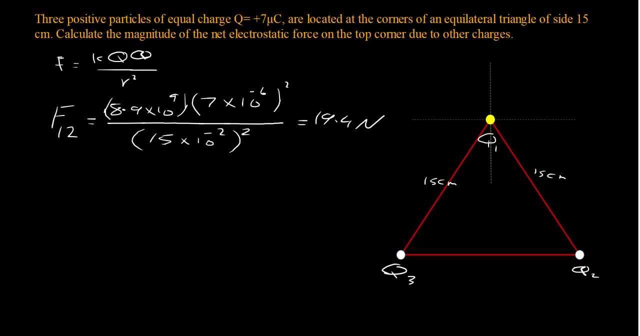 let's try to draw the- Okay, Okay, All right- direction of this electrostatic force. so I'll take the green now. all charges are positive, so this is a positive charge and also this one is a positive charge. now, because they are both positive, their force will be repulsive and it will be. 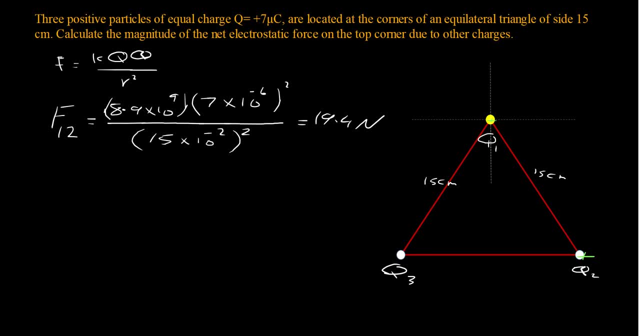 as an extension to the line connecting both forces, both charges. sorry, so that will be the direction of F 1, 2, which is repulsive. all right now to find out how much is the force generated on charge 1 because of 3? amazingly, it will be the. 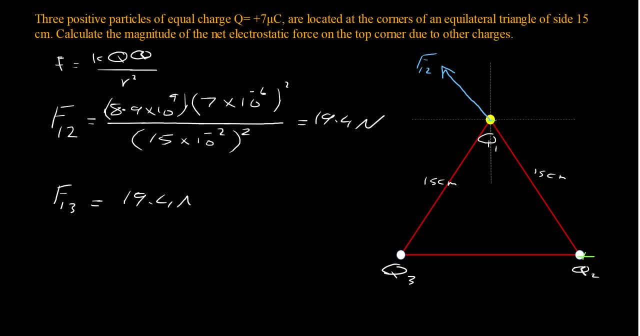 same value. it's 19.4 Newton. why? because it's the same magnitude charge and it's the same distance between the Q 3 and Q 1 as Q 2 and Q 1, so I will have the same magnitude of the electrostatic force. now 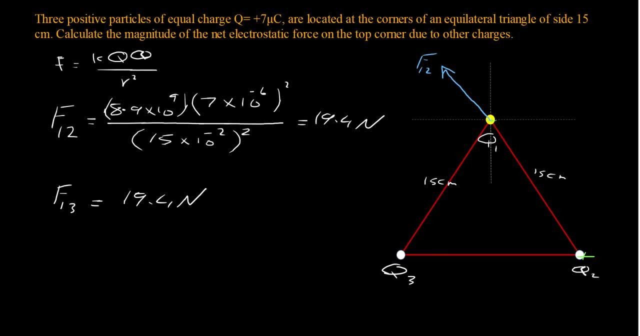 let's draw the direction once again. I will have all positive charges that will generate a repulsive and will be an extension from our target. here it is. that's our F 1- 3. okay, cool. now this is not the net electrostatic force. we have to analyze our two forces vectors into two components. so let's 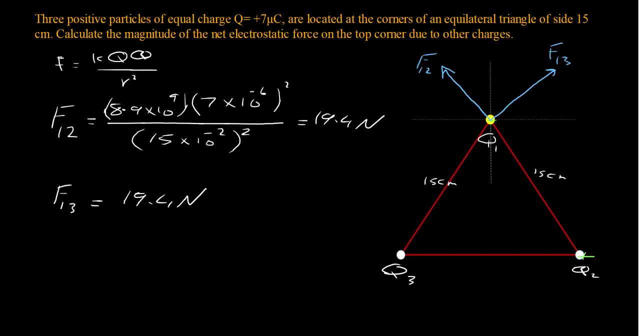 start the fact that I have an angle here. I will call it alpha and I'll call this one beta, and because it's an equilateral triangle, I know this is a total 60 degrees, which means alpha and beta. they will share that 60 degrees equally so. 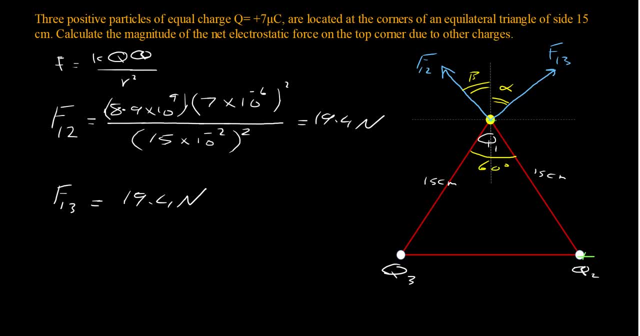 30 degrees. so let's try doing the analysis, analyzing our components. sorry, that will be F 1- 3 sine alpha, and I will have one here for F 1- 3 cosine alpha. okay, let's pick another color for F 1- 2. I will have here F 1- 2. the force on 1. 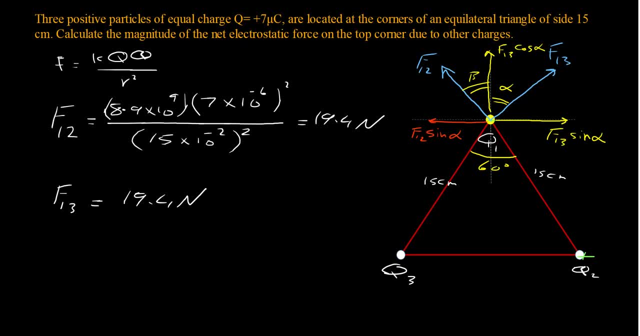 because of 2 sine beta. sorry, let's erase this one. make it more clear that is should be sine beta and same here. I will have the same direction as well. top F: 1 the force on 1 because of 2 cosine beta. okay, if we want to try that. 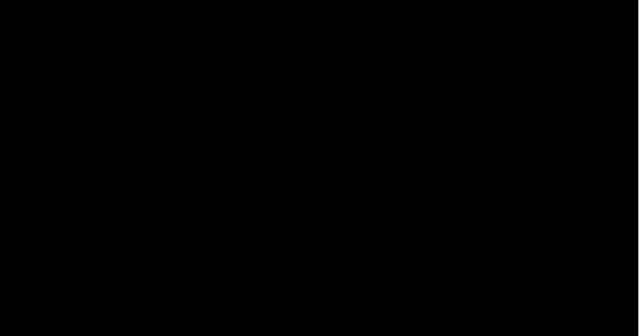 in more clear. I can do it this way. so this is my charge, the yellow one, it's located here. now what we said. I will have the force generated here. now what we said. I will have the force generated by the third charge on 1 with a sine alpha, and also I have opposite to it, the 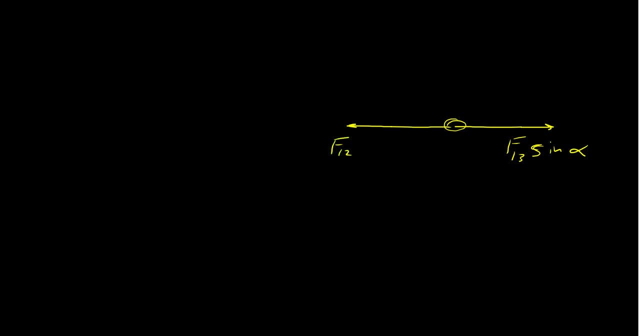 force on 1 because of 2 sine beta. now look at the color. I have. two forces went up to components and it will be 1, 3 cosine alpha, and also I would have F 1, 2 cosine beta. okay now, because the magnitude of the forces 1 & 3, 1, 2 & 1, 3, & F 1- 2 equal F 1, 3 and alpha equal sqrt beta. they both, therefore, are equal. F 1, 2 cosine F 1, 3 now because the magnitude of the forces 1 & 3, 1, 2 & 1, 3, F 1, 3, and also I will have F 1, 2 cosine Sqrt Peta. okay, now because the magnitude of the force 1 and 3, 1, 2 & 1, Trugue 2, equal Sqrt Peta and a. 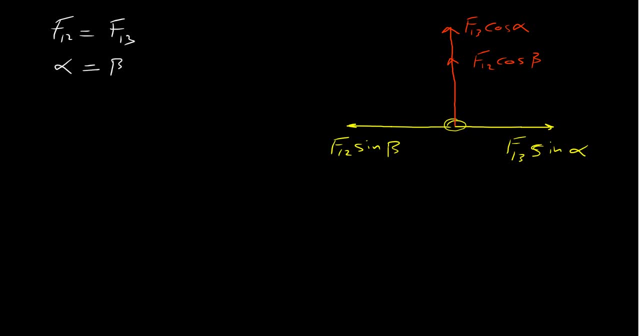 and alpha equal beta, they both 30 degrees. let's make it really easy to find how much the total electrostatic force in the x-axis. in fact it will be zero because simply these they will cancel each other. the equal in magnitude opposite n direction. but for the y-axis,